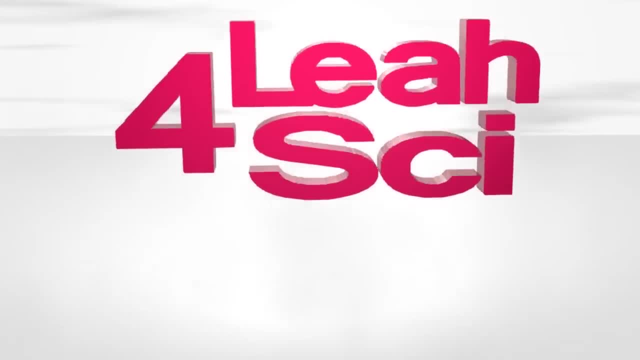 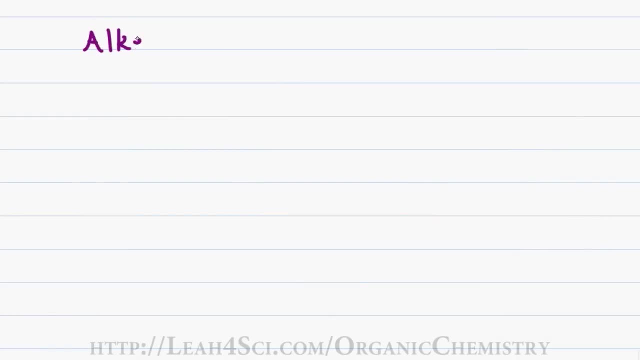 Leah here from leah4scicom, and in this video I will show you how to name a molecule that has both an alkene and an alkyne. Recall that an alkene is a molecule that has a carbon to carbon double bond and gets the last name of ene, and an alkyne is a molecule that has 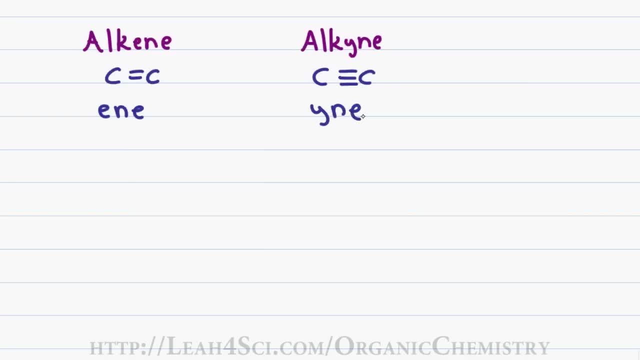 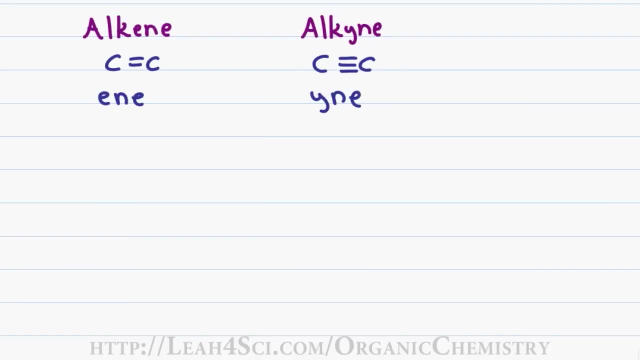 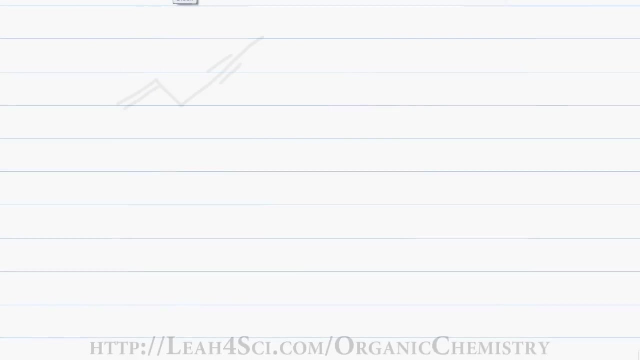 a carbon to carbon triple bond and gets the last name of ein. But how do you name a molecule that has both a double bond and a triple bond? An alkene and alkyne can exist in the same molecule and you prioritize based on where each functional group shows up. We'll use 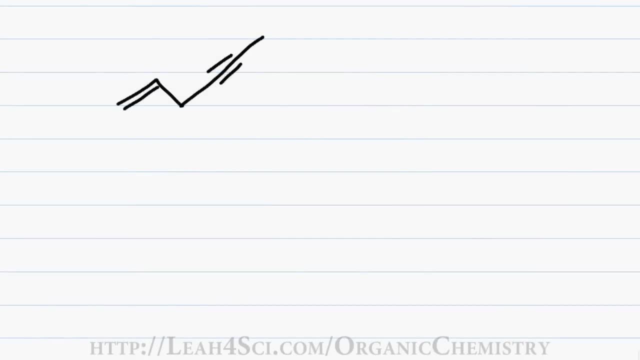 this molecule as our first example. since I only have one long chain, I highlight my parent chain and then decide how to number. I have the option of numbering from the left, giving me a one for the double bond, or numbering from the right, giving me a two for the triple. 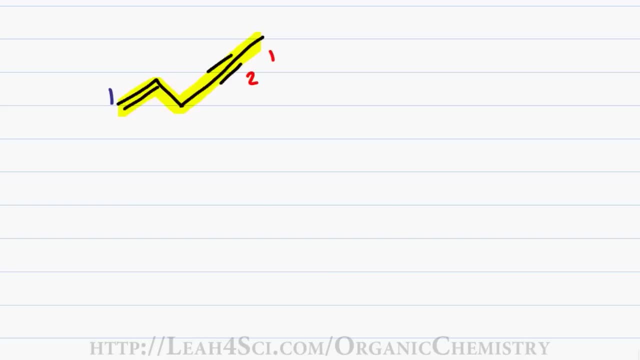 bond. The priority here is determined by which functional group of the molecule that has the double bond and a triple bond. I have group you hit first, and so I have to number from the left because I have number one, which is lower than two. Having six carbons in my chain gives me a first name of hex Having 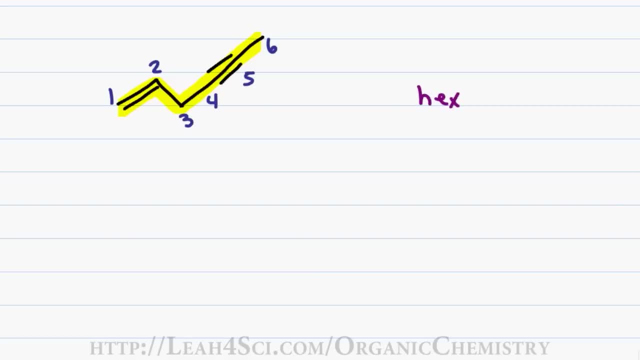 both a double and a triple bond. I get two last names for this molecule. I get a one, ene, for the double bond and a four ein for the triple bond. When it comes to putting the molecule together, ene gets a higher priority than ein in the naming, and that is because 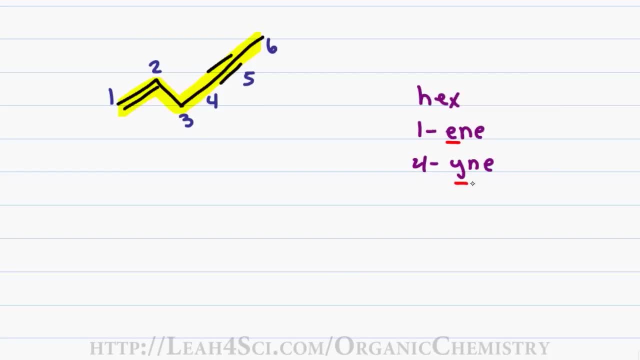 in alphabetical order, e comes before y. In previous examples we've shown that you could put the number before the name, but because we have two last names here, each number has to proceed its specific functional group. This gives me a complete name of hex one ene. 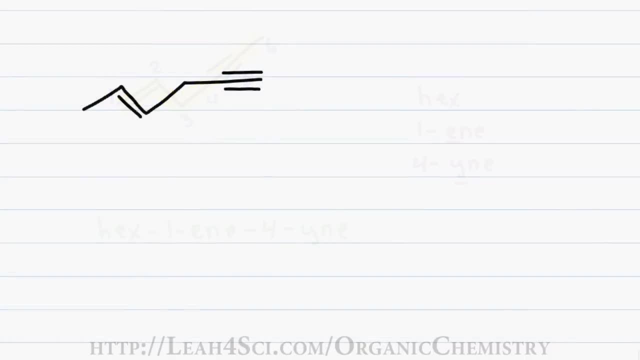 for ein. In this example, I switched the order of the substituents so that once again we have a straight chain with an alkene and an alkyne, but in this molecule, since the alkyne is terminal, the alkyne gets priority for numbering, and so I number, starting from the right Once. 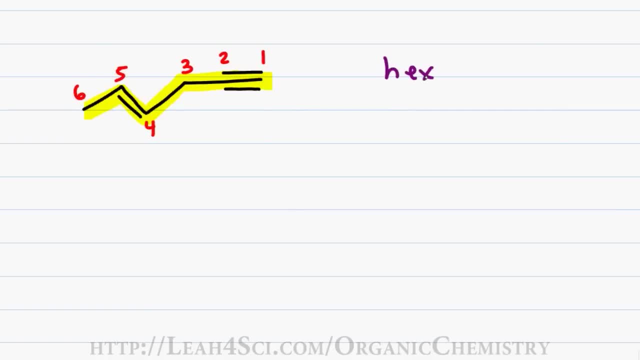 again, six carbons gives me a first name of hex, and the double bond and triple bond give me a last name of both one ein and four ene. In this case, even though the triple bond has higher priority for numbering e comes before y, and so ene still comes before ein. 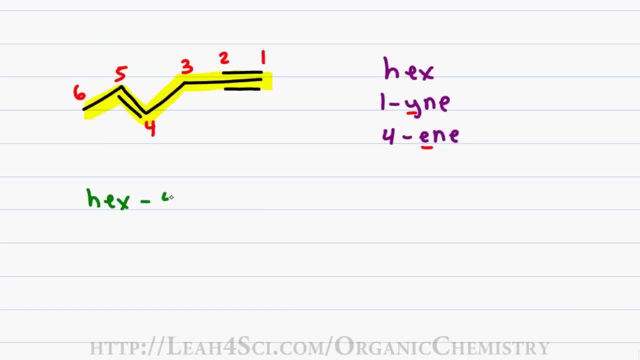 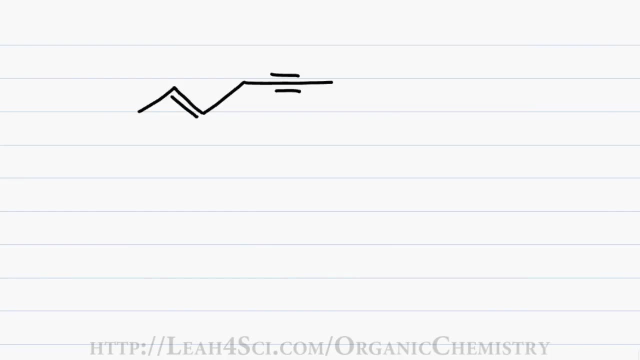 in the name, and so the molecule is named hex four ein one ein. Now what happens if I have an example that potentially gives the alkene and the alkyne the same name? Once again, I start by highlighting my pairing chain, But now I have the option of numbering. 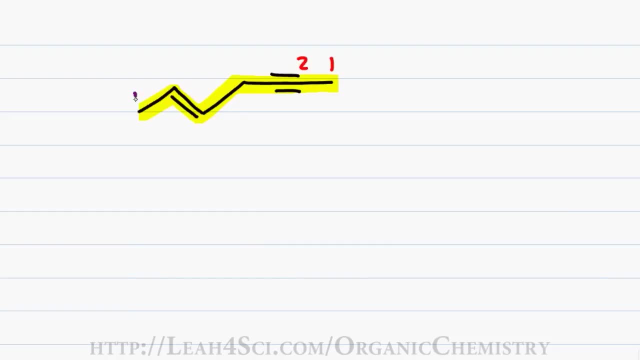 from the right, giving the triple bond the number two, or numbering from the left, giving the double bond the number two. In this situation, the alkene has the higher priority than the alkyne, and so we start numbering from the left. Having seven carbons in my molecule, 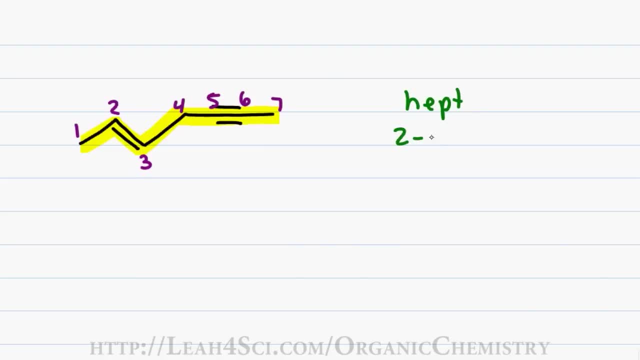 gives me a first name of hept. Having this first name will represent the first name of the molecule. Now, if I always consider all of these by numbering from the left, this- Having both an alkene and an alkyne- gives me the last name of 2-ene, and another last. 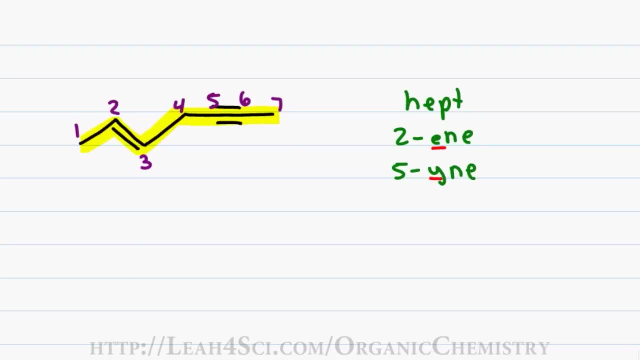 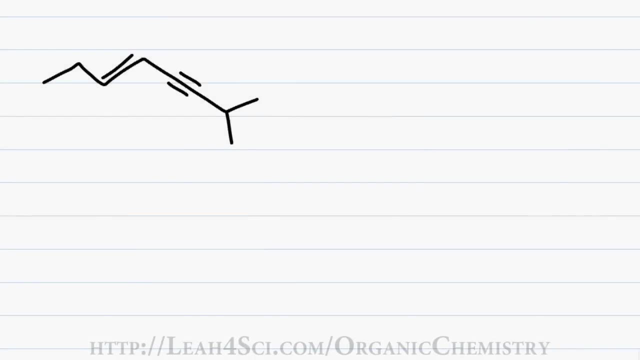 name of 5-ine. Since E comes before Y, I get a final name of hept-2-ene-5-ine. Now let's look at this example. The first thing I do is highlight my parent chain and determine which way to number. 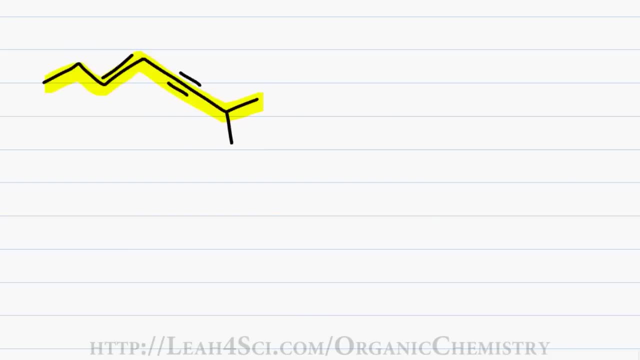 Going back to the standard IUPAC rules, you have to number the chain so that the substituent gets the lowest number. In this case, I have to start numbering from the right, because I have a methyl group on the second carbon. Now let's put the name together. 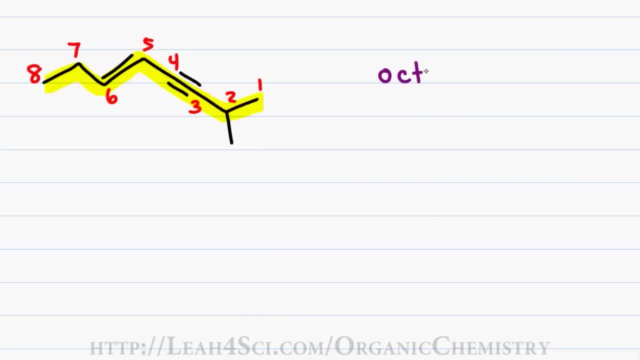 I have 8 carbons, giving me a first name of oct. I have a double bond on carbon 5, giving me a last name of 5-ene. I also have a triple bond on 3, giving me a second last name of 3-ine. and then we have 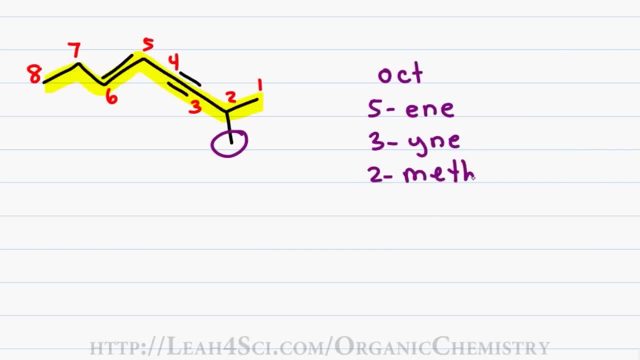 a methyl group on carbon 2, giving me the prefix 2-methyl When putting this molecule together, Methyl is your only carbon. It's your only substituent. therefore, it's your prefix. Ene and ein are both your last names and sorted in alphabetical order. 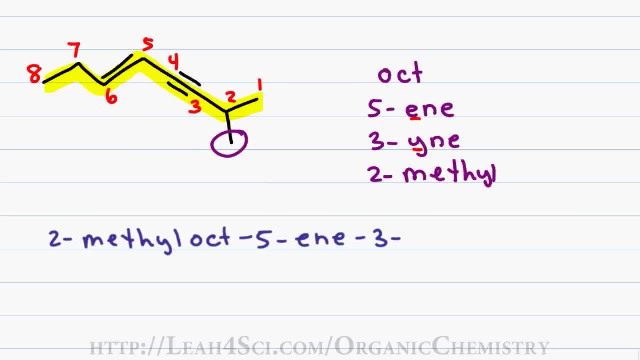 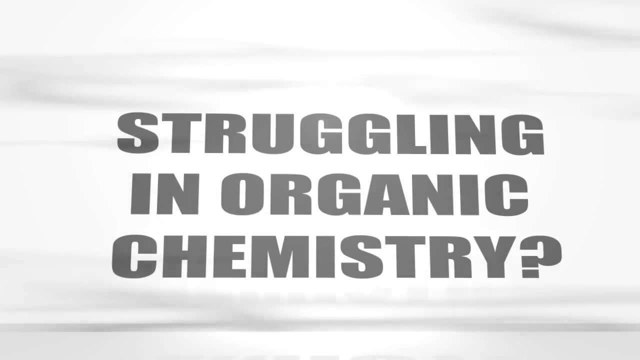 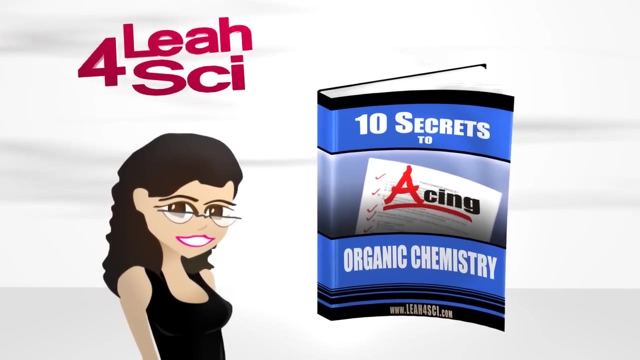 This gives me a final name of 2-methyl-oct-5-ene-3-ine. Are you struggling with organic chemistry? Are you looking for information to guide you through the course and help you succeed? If so, download my eBook 10 Secrets to Acing Organic Chemistry using the link below or: